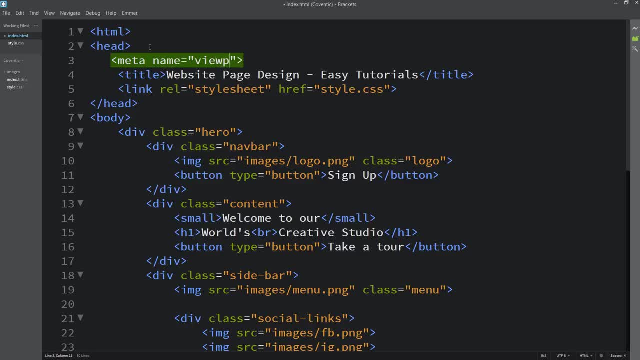 I am adding meta name: viewport, Then content equal to width, equal to device width, then comma space, initial scale equal to 1.. You need to add this tag in your html file in the hit tag. After that, again, I will refresh the website. You can see some changes on this website. 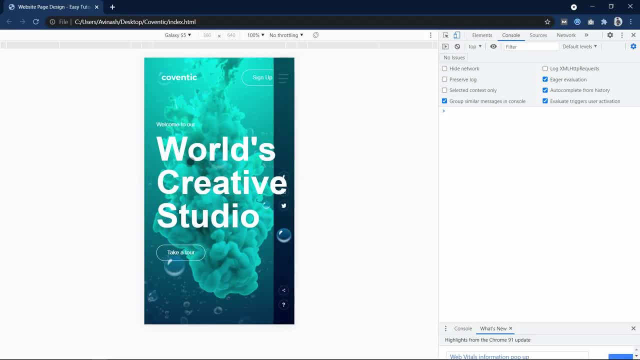 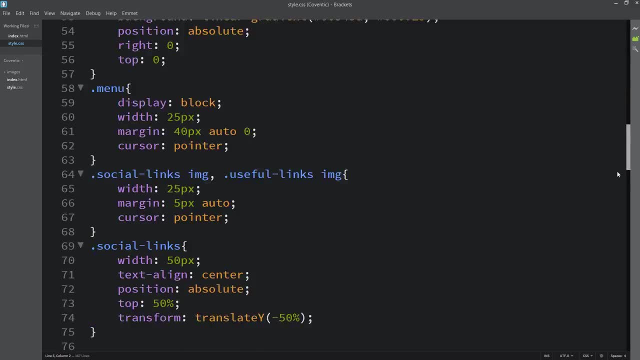 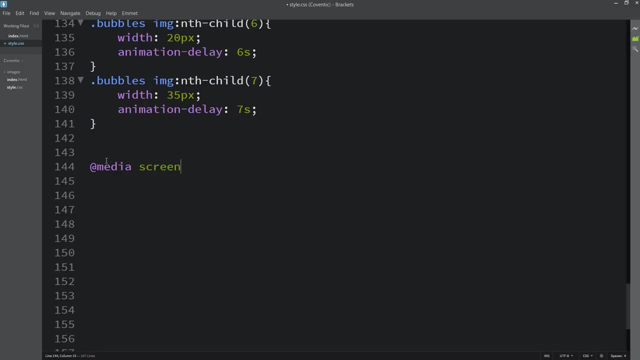 You can see this text is looking very big on this small screen. So we have to reduce the size for this text in the small screen. So just come back to the css file and let me scroll down and here we will add media Screen and in this media we will add the condition: 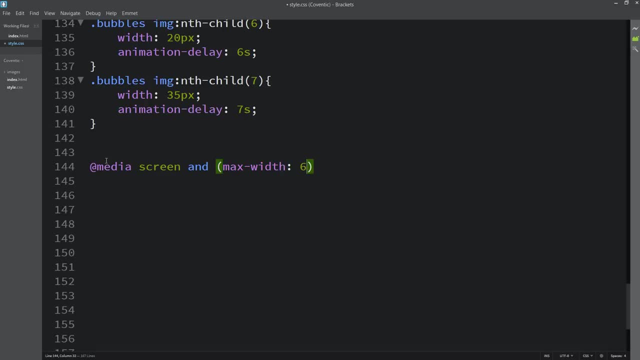 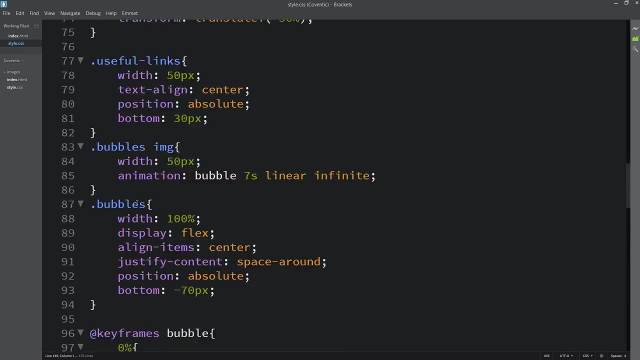 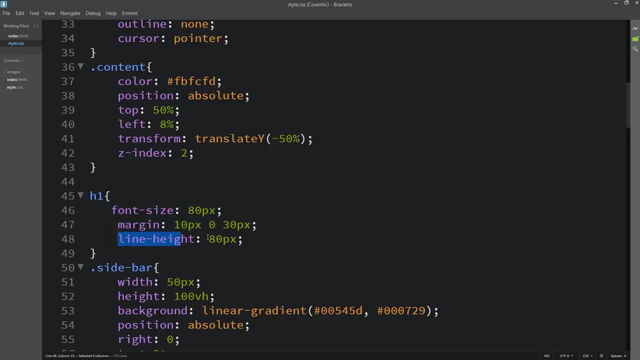 So the condition I am adding: max width equal to 600.. So in this media we will add some css properties. That css will be applicable for the small device. Device width should be 0 to 600 pixel. So let's come back to the top and here you can see I have added this h1 for the title. 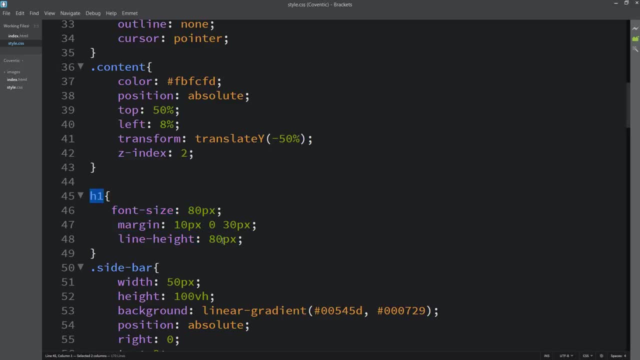 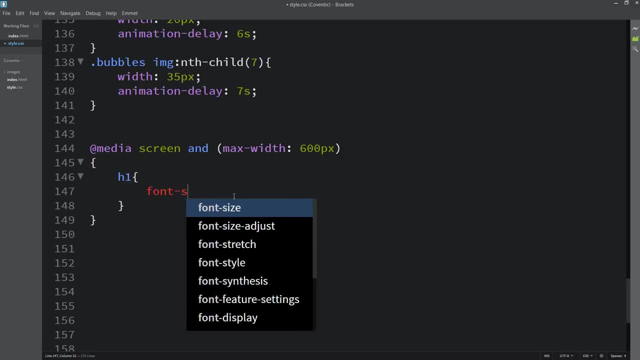 and here we have the font size and line height. So we have to reduce this one. So just copy h1, write it here in this media. Here we will add font size 36 pixel and line height 50 pixel. So we have decreased the font size and line height. 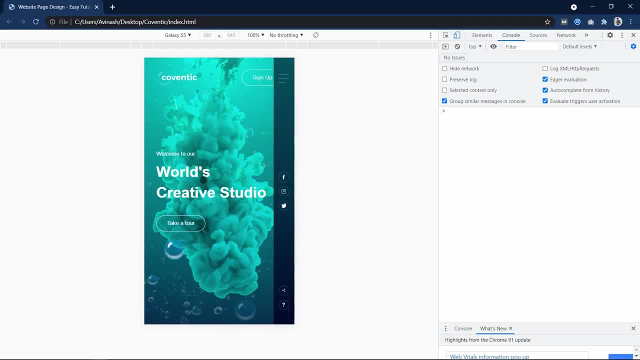 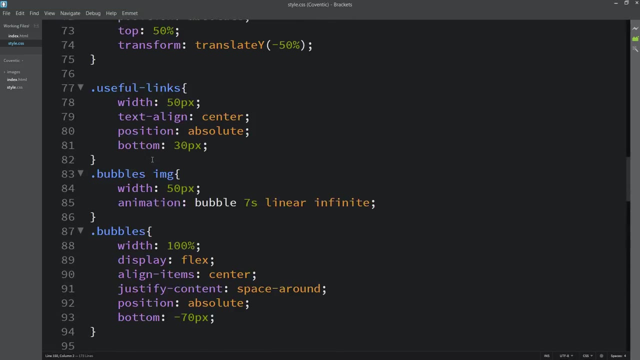 Now you can see the font size is perfect for this device size. After that, you can see this vertical sidebar on the right side. So we will move this Vertical sidebar to the bottom and it will be horizontal. So for that, let's come back to the css file again. 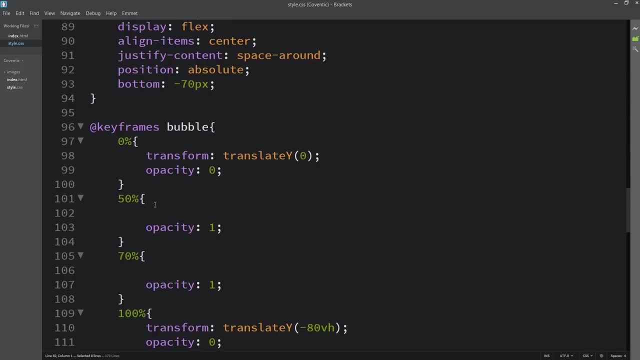 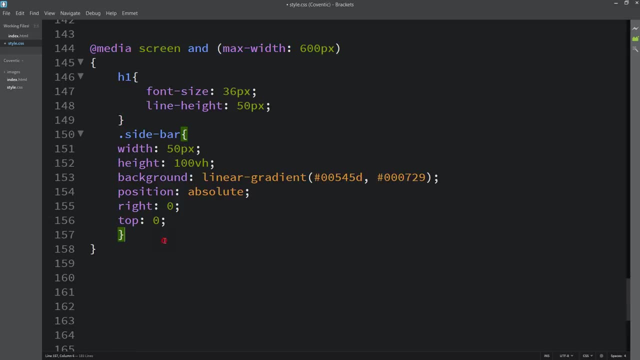 Here we have the css for the sidebar, So let me copy the complete css and add it here in this media. for the smaller screen: Here you can see we have added width 50 pixel. So now we will change the width 100%. From the left to right it will be 100%. 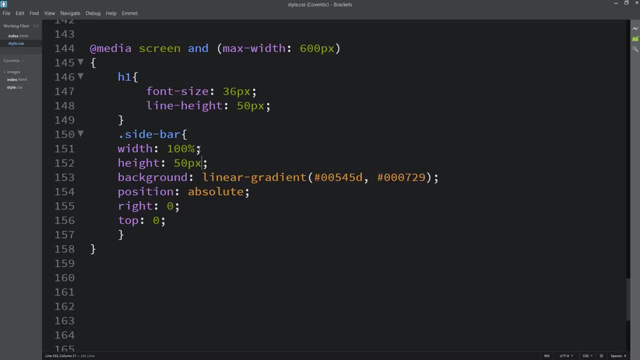 Then height, So we will add the height 50 pixel and we will not change the background. So remove this one. We will not change the position. Remove this one and right, it is already there. So let's remove this. and instead of this top 0 we will add top auto and here we will add: 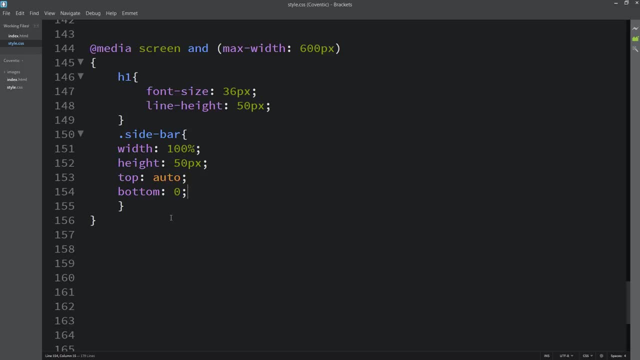 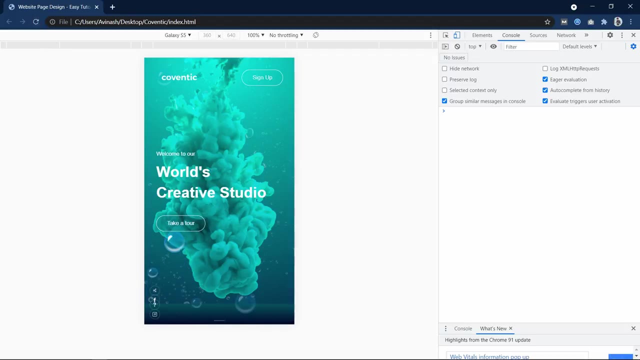 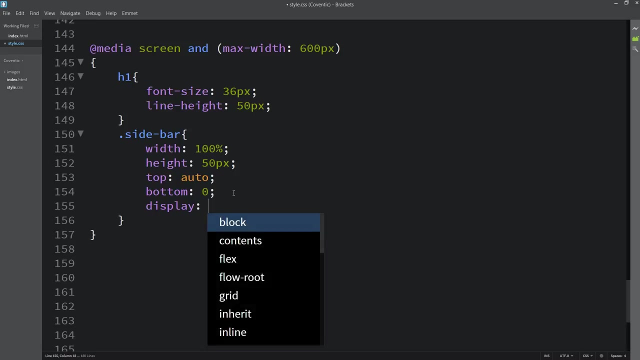 bottom 0.. So it will come at the bottom. After applying this, you can see this section is coming at the bottom, But these icons in the left side. So let's come back and here we will add display, flex, align items, center and justify content. 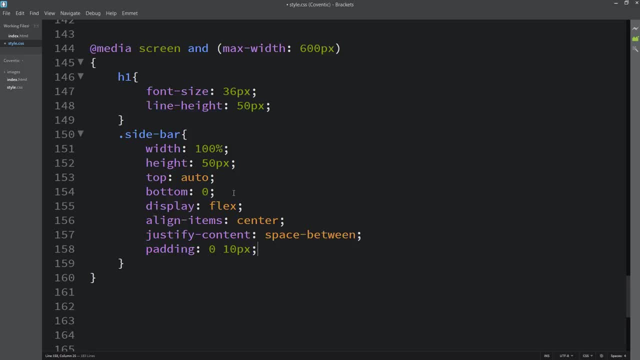 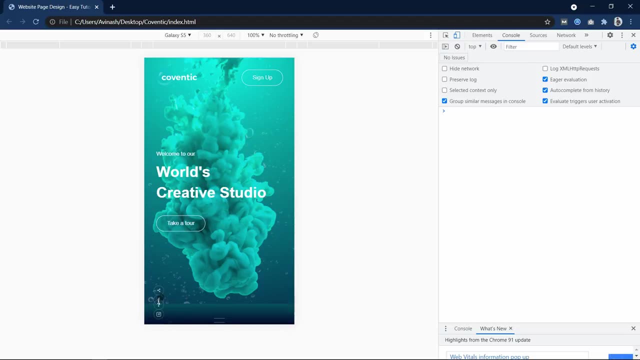 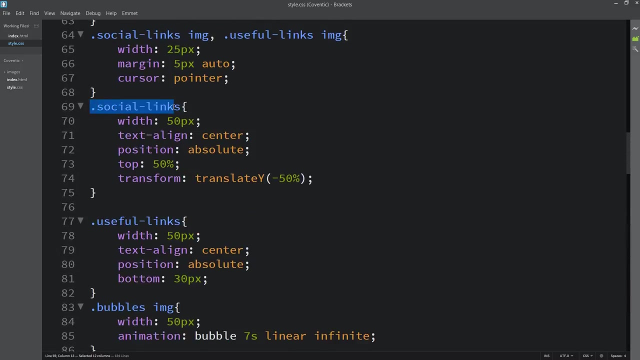 space between and we will add some padding and box sizing will be border box After that. still, you can see there is no changes in this icon because we have added some position. I think You can see In this social links and useful links- we have the position absolute. 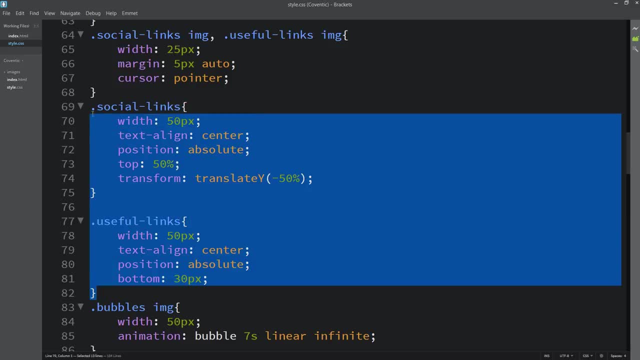 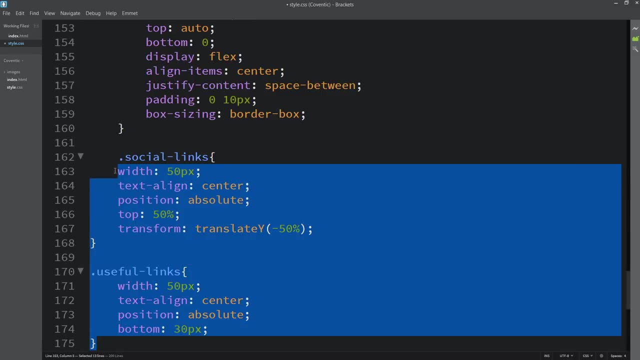 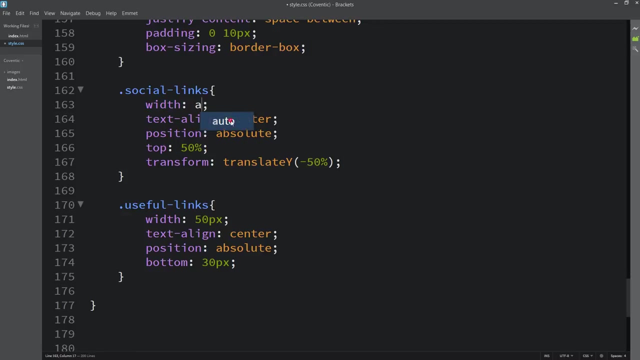 So we have to remove this absolute for the small screen. So just copy these css and come to the media portion. Add it here in this media and let's change the css here in this social links: Here we will change the width auto, Then remove this text align. 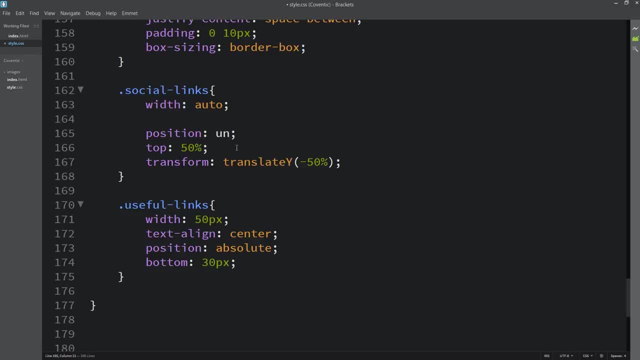 And instead of this absolute we will add position unset, And here we will change the width auto. Then remove this text align, Remove this top and this transform. we will make it none. So there will be no transform Now in this one also, we will add the width auto. 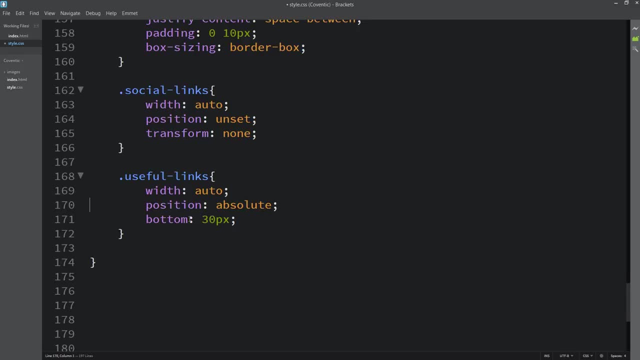 Remove this text. align Position will be unset. Remove this bottom. That's it. After applying this, you can see some changes in this icon. Now we have to set the css for this menu icon. So just come back and let's see where we have the css here. 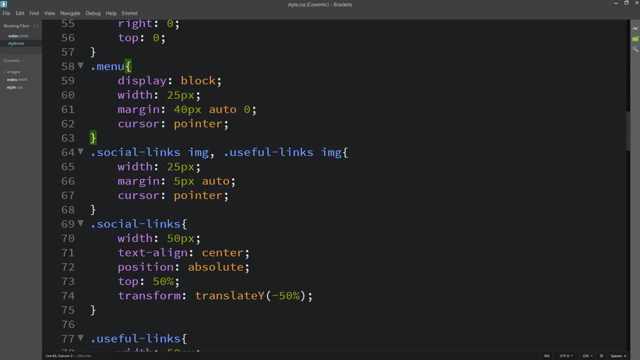 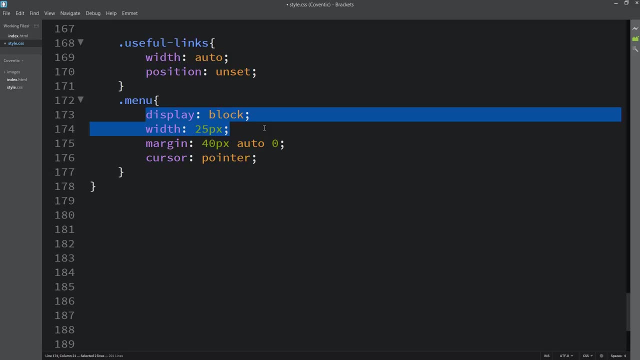 Here is the css for the menu icon. Copy this one And add it here in this media. Now, here we will change the width, So width will be 18px. We will change the margin 0.. That's it, And after that again refresh the website. 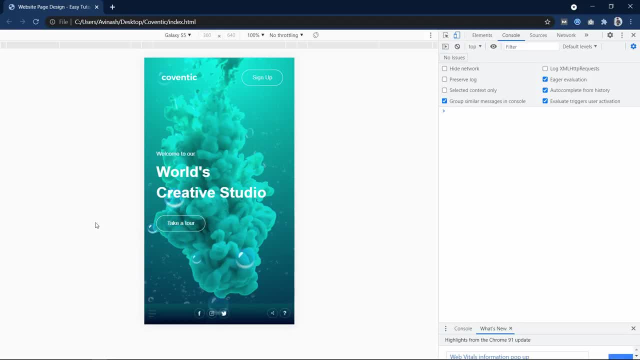 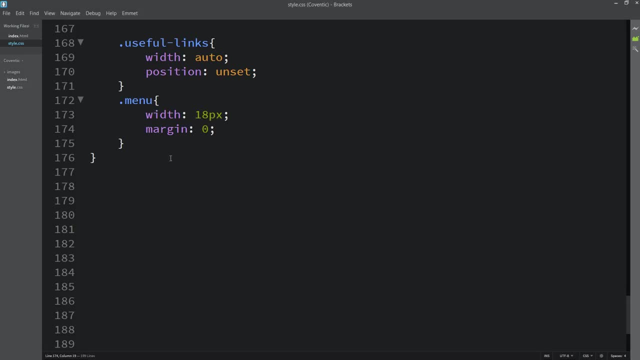 You can see the bottom. It is looking good, So we have changed this one also. Next we will change the background. You can see the background image is so much zoom in, So let's see we have this hero here And here we have added the background image. 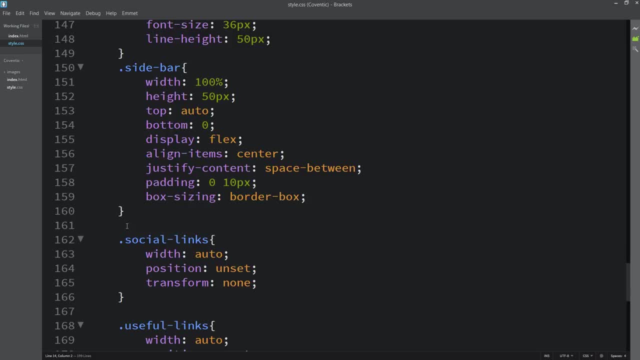 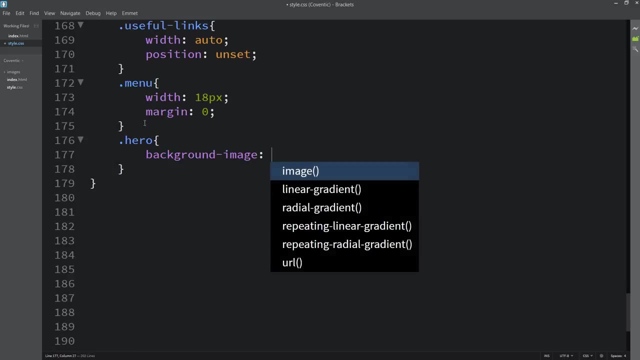 So let's come back to the media. In this media query we will add the class name hero, And here let's add one background image. Here we will add the linear gradient color. So linear gradient. Then first color code And I will add the second color code. 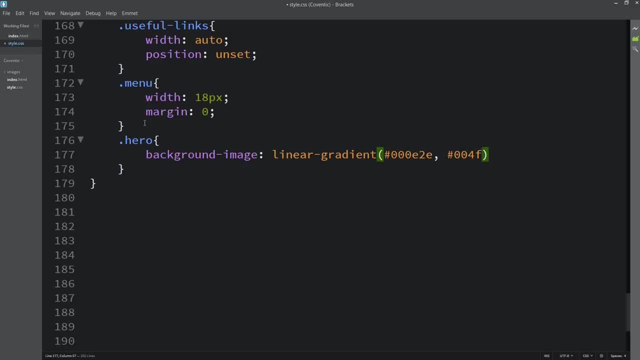 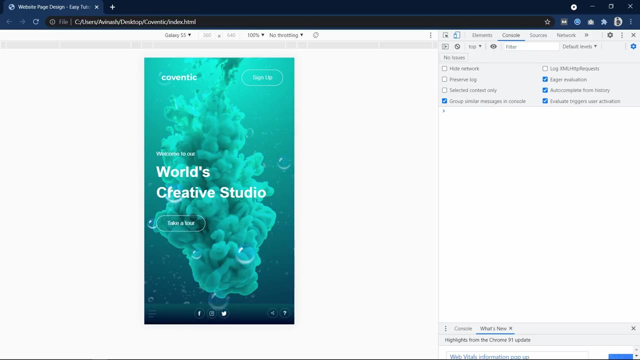 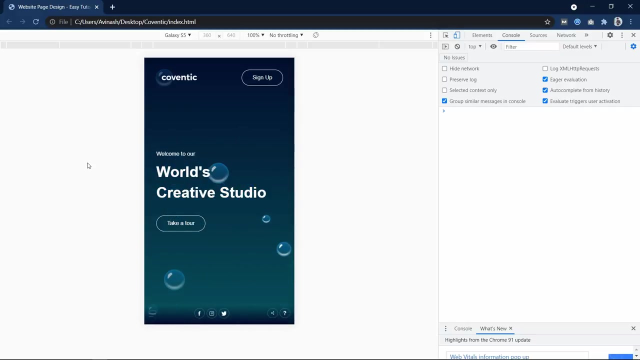 So in this way we can change the background for the different device size. After adding this, if I refresh the website, you can see the background is a plain linear gradient color. There is no image in the background. Suppose you have an another image that also you can add for the small screen. 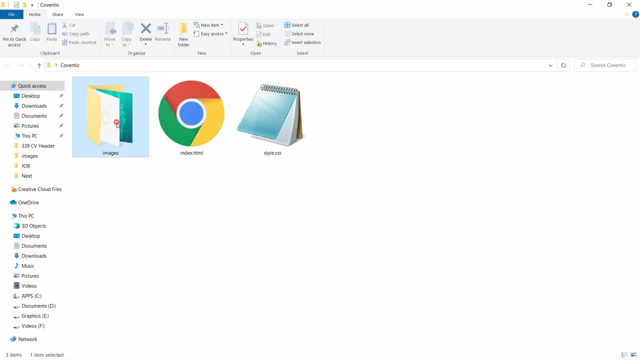 So let me come back And here in this folder you can see, I have one another image here. It is a vertical image which is perfect for the small screen, And it was the original image which is displaying in the full screen, But we will use this vertical image. 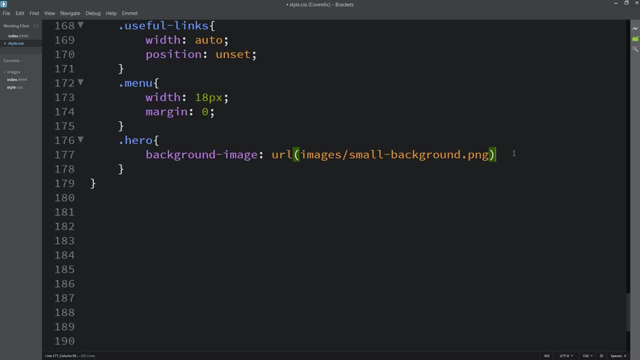 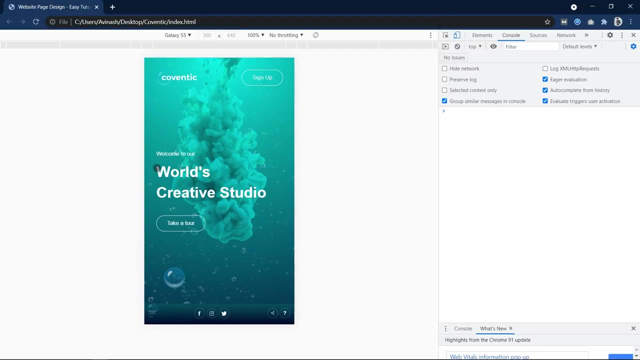 So here let's add url image file path Like this: And after applying this, refresh the website again And you can see the different image for the small device. Now this web page is looking good for the mobile device. Now I will tell you. if you want to add something different, css for the other device size. 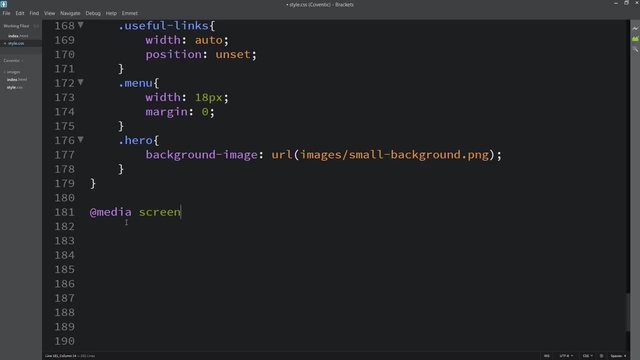 Suppose you want to add different css for tablets. So how to write the css media query for the tablet? We will add media screen and, and here let's add max width, It will be 900.. And again add min width: 600.. Okay, 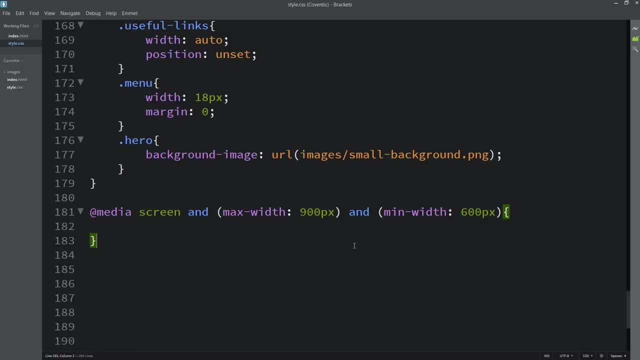 So what happened? Okay, So whatever css properties we will add in this media, That will be only applicable for the device having width between 600px to the 900px. So this is how you can use css media query to make any website responsive.